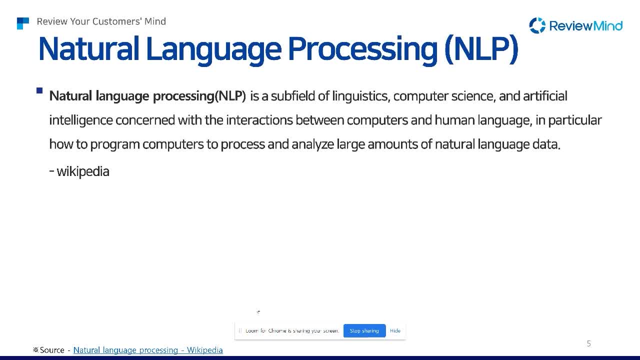 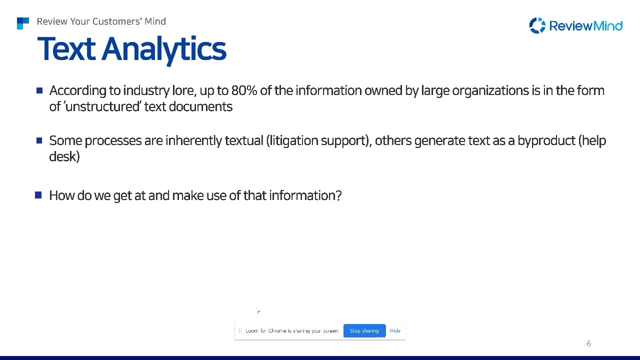 with the interaction between computers and human language, in particular how to program computers to process and analyze a large amount of natural language data. To get a more simple understanding, I just can say that NLP is all about how do we get those text data and 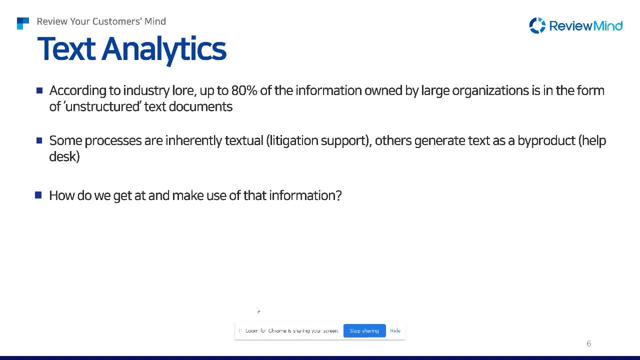 make them useful in a way to interact with computers and machines. Traditionally, this NLP is a tool that can be used to analyze a large amount of natural language data. To get a more simple understanding, I just can say that NLP is all about. how do we get those? 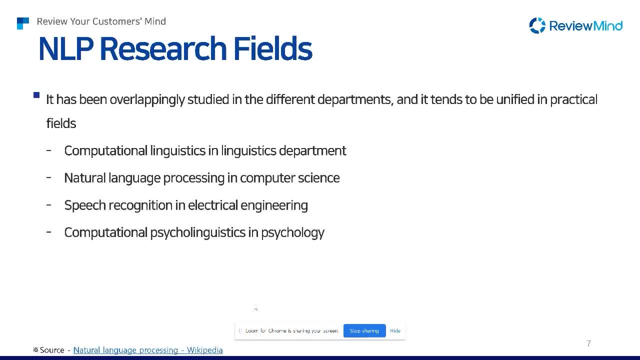 text data and make them useful in a way to interact with computers and machines. Traditionally, this NLP area has been studied in many different departments, such as in computational linguistics departments, in computer science departments or speech recognition in electronic engineering. 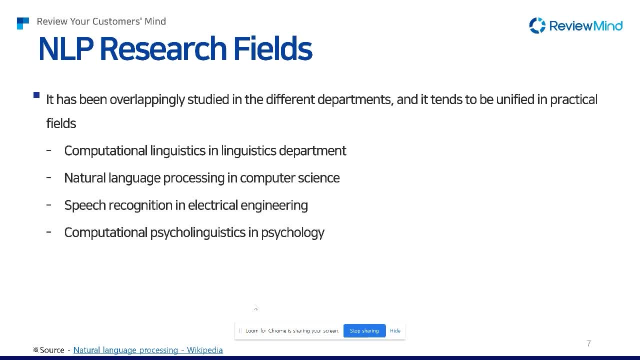 etc. But nowadays it tends to be unified as a conversion technology so you can see the product like Alexa or Google Nest. So in modern NLP field, NLP is a tool that can be used to analyze a large amount of natural intelligence. To get a more simple understanding, I just can say that NLP is all about how to. get those text data and make them useful in a way to interact with computers and machines. Traditionally, this NLP area has been studied in many different departments, such as internet tools, web applications and chat games. I just can say that NLP is all about how do 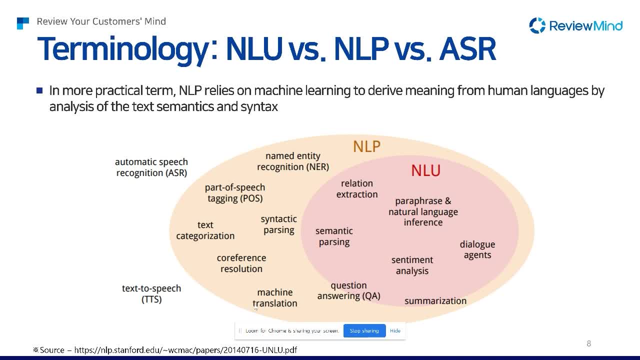 we get those text data and make them useful in a way to interact with computer science, spectrometry, whether in VMware or Tableau technology. In this context, simply put, NLP is more related with the synthetic aspect of language analytics. meanwhile, NLU is more related with the semantic aspect of 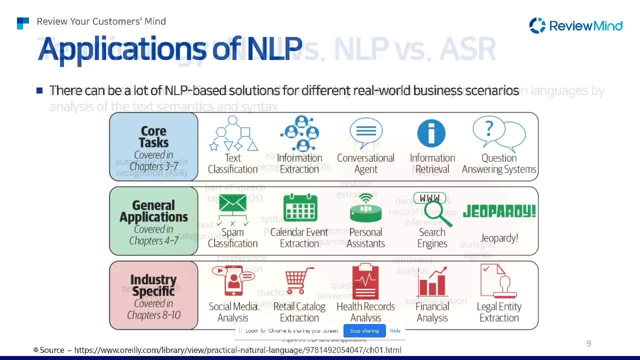 Virginia, Thank you of language analytics. Next, let's see the applications of an NLP. these days There can be a lot of dynamic solutions for different real-world business scenario. Several of them here must be familiar with you already: Search engine and spam classification. 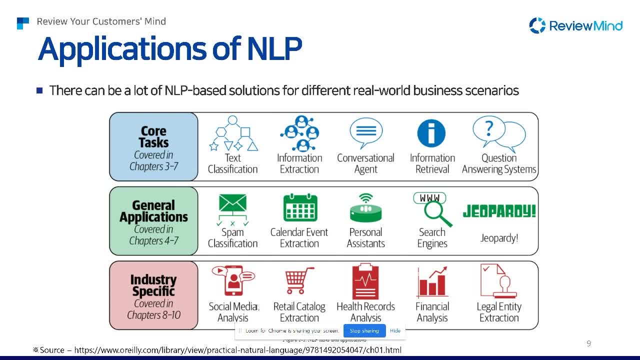 maybe you are using them in your everyday life. Meanwhile, conversational agents like chatbot or automatic Q&A answering machines are getting more and more popular. The company like us, ReviewMind. we are focusing on semantic analytics on people's comments like review social media community posting. 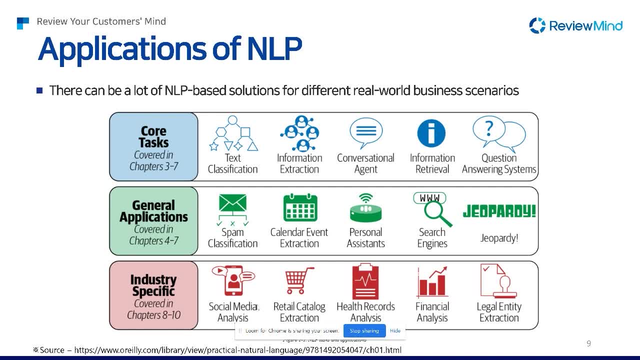 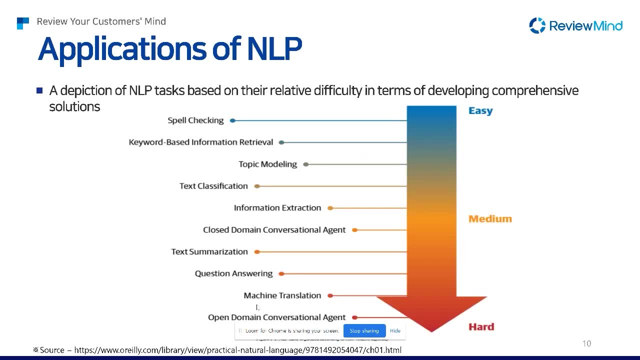 However, I think these technologies are still working on the baby step, especially in their application lines, which means there still exists a lot of innovation points with intensive analytics. So let's take a look at some of the new technologies that are coming out of the R&D process. 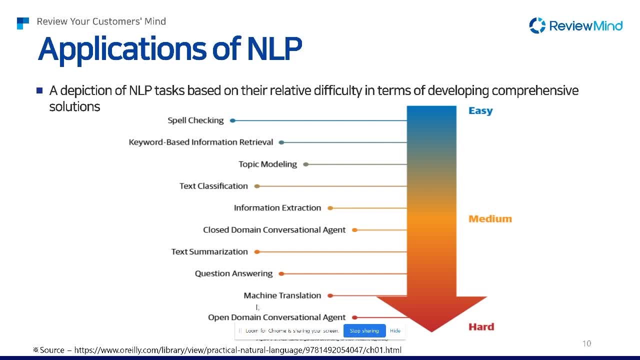 So in here you can check the technical maturity in all of each NLP task. For example, spell checking technology is quite mature in English, even though it depends on which language you are targeting at. Definitely for English. there are many options. 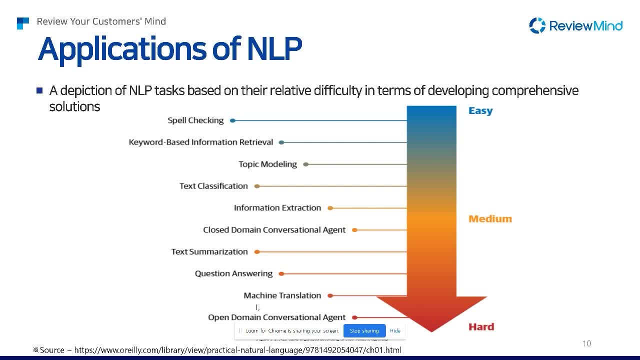 for spell checking, and they are quite great. Meanwhile, for Korean, there are a few options, but we will talk more about them in this video. So let's get started. So let's start with the NLP basics. NLP is a very basic technology. 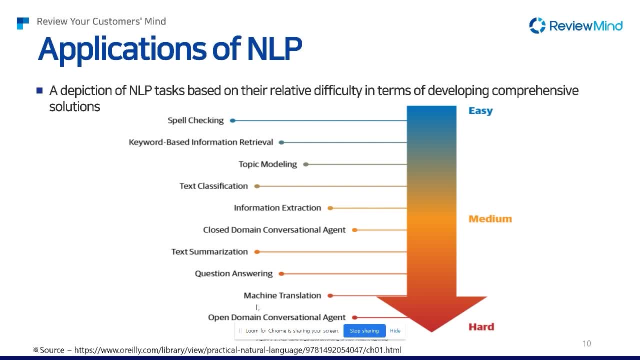 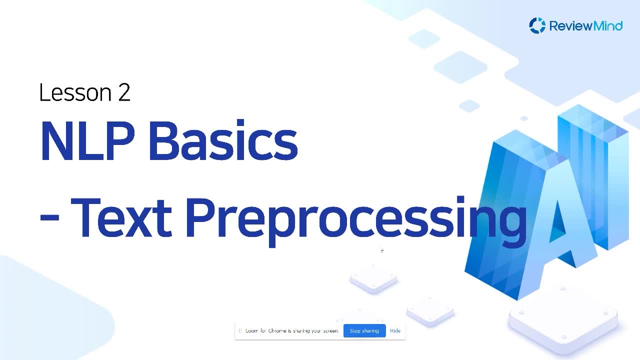 and it is not only for Korean, but also for other languages, It is also for English, and it is also for Thai, and it is also for Chinese, and it is a very basic technology. so we will talk about it later, but for this we will talk about NLP basics. 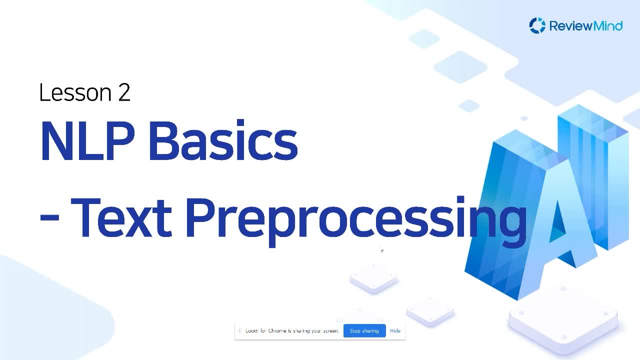 at a later stage, and we will also talk about how to make it work for a computer to understand low text data. So let's start with the basics. So let's start with the basics. Usually you have heard that the data processing phase is usually very time and labor consuming. 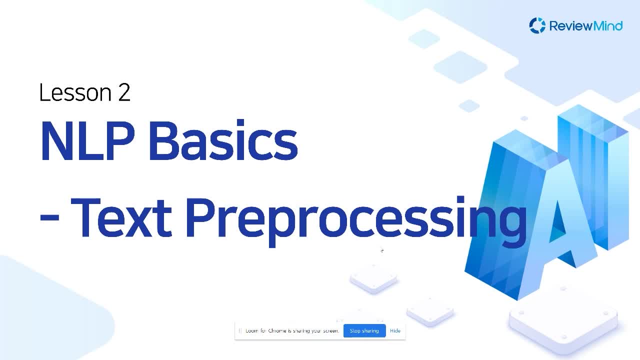 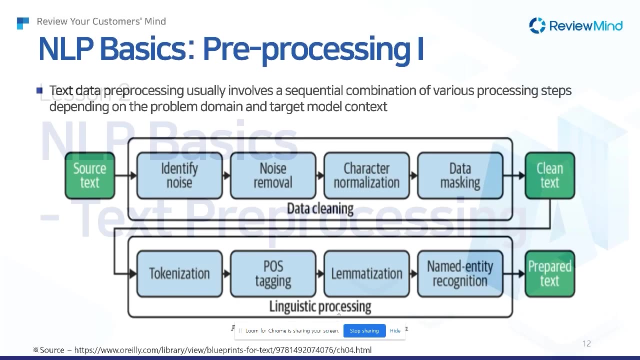 but at the same time very critical for the whole machine learning analytic process, And it is so in the NLP area. with text data, It can involve many tedious but delicate procedures, depending on what kind of model problem you are targeting. Text data processing usually involves a sequential combination of various preprocessing steps. 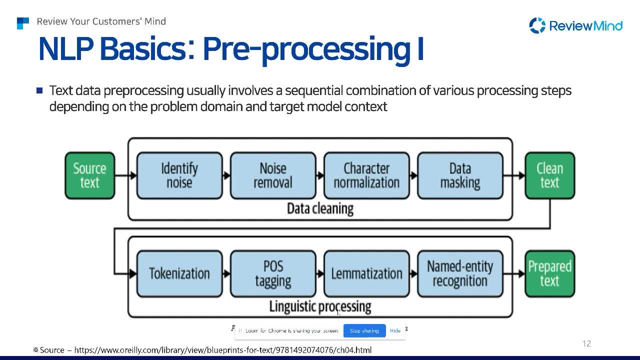 depending on the problem domain and target model context, It can be roughly divided into two parts. as you see this diagram, The first text clean part is including identifying noise, removing those noise, character normalization, data masking, etc. Usually we identify punctuation. 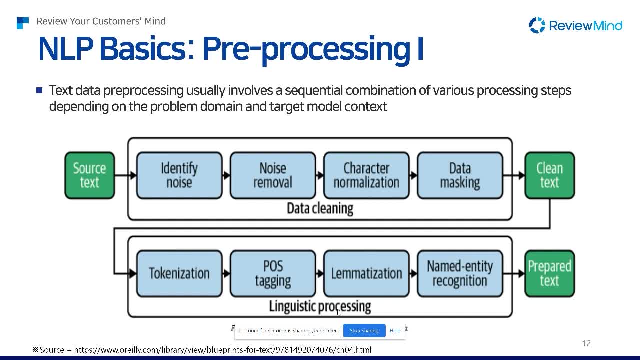 stop word numbers as noise. However, depending on your target model, problem numbers can be a very important factor you should not remove. In other case, in the semi-structured text documents like financial audit reports or a legal document form, those structured text template parts can be treated as a noise. 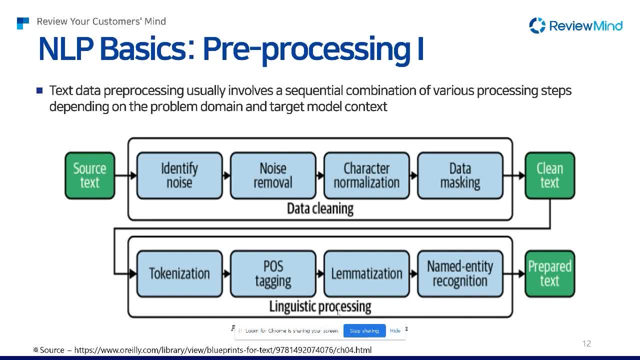 too, as you should remove So like this. you had better carefully consider processes unnecessarily on your target domain rather than apply one universal combination of text preprocessing techniques to all the situations. Character normalization: you change uppercase into lowercase, especially in English-like. 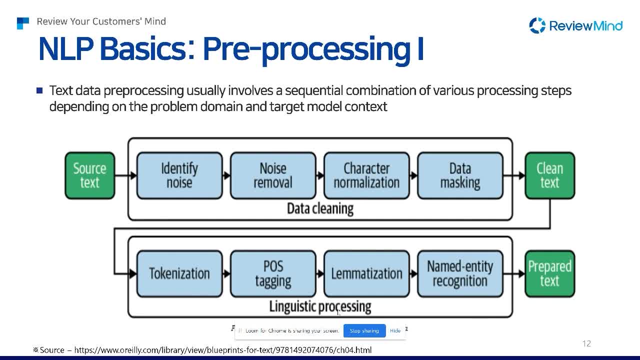 languages because computers understand upper and lower differently, unlike human beings. Data masking is also important these days as personal information such as phone number addresses those should be removed- or data masking for their privacy protection. Sometimes this can be used for prephrasing issues in text, analytics and the other linguistic. 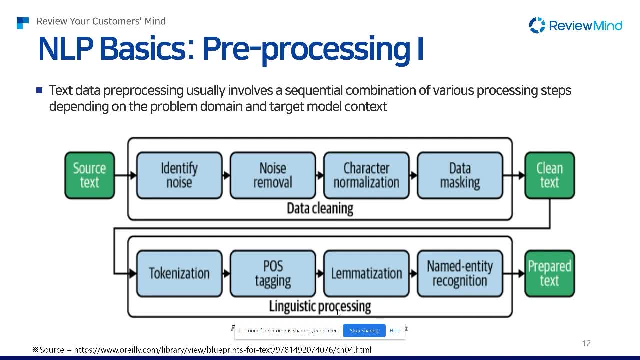 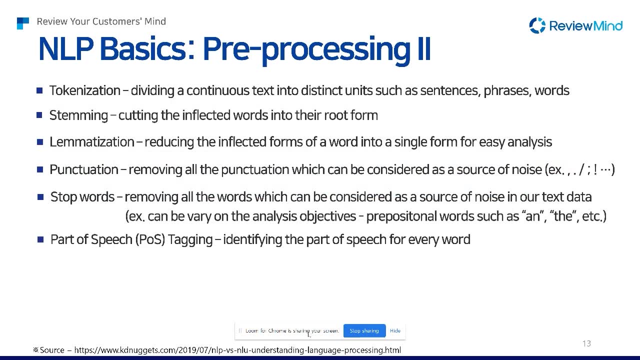 processing parts include tokenization, stemming or lemmatization, POS tagging, etc. These are the results to try to understand the text in more deep level. So in this session we will discuss these general text preprocessing tasks one by one. 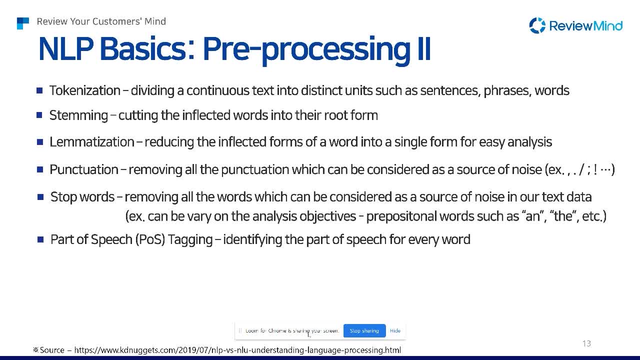 and we'll see the example use cases with actual Python code using tools. So, as a basic NLP preprocessing task, we will talk about tokenization, stemming and lemmatization, removing punctuation and subwords, And we will also talk about the general text preprocessing tasks. 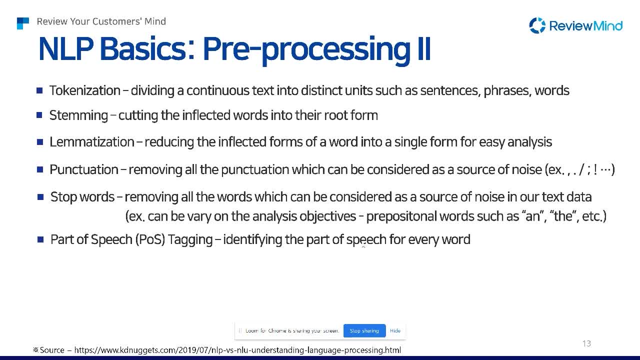 So, as a basic NLP preprocessing task, we will talk about tokenization, stemming and lemmatization and POS tagging. Okay, before we go to the use cases of each text preprocessing task, let's talk about the tools to help us to handle these NLP tasks. 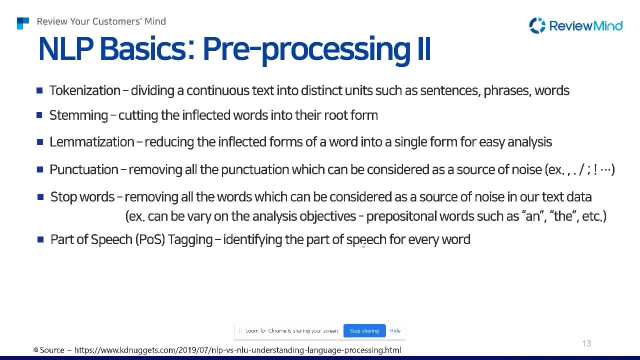 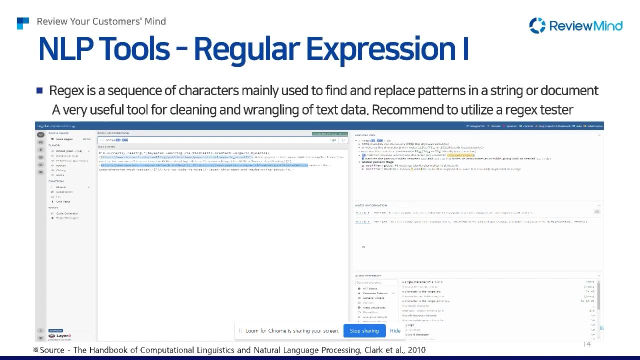 There are many tools out there, but I would like to mention the most popular and representative tool, which is regular expression, NATK and spaCy. Regular expression is a sequence of characters mainly used to find and replace patterns in a string or text. 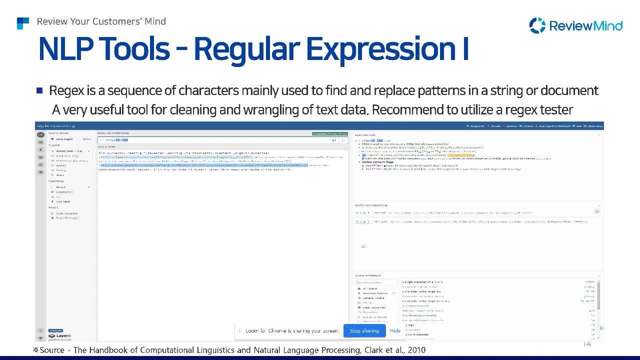 It is a very useful tool for cleaning and wrangling of text data. For practical purpose, I recommend you using text tester, regular expression tester. It's free and convenient to check the complex regular expression based on your target data set. Actual execution of regular expressions is very simple. 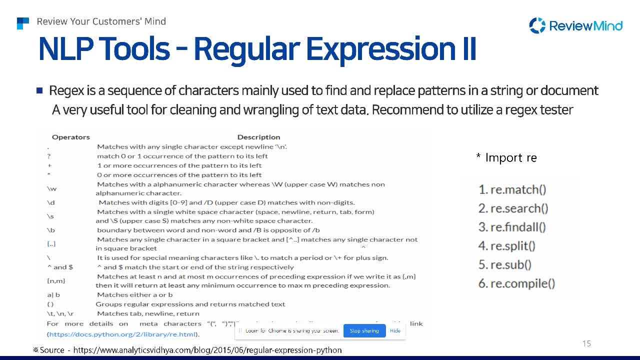 You just need to run the test. You just need to run the test. You can simply use a Python built-in package. Its name is re. This is the most commonly used tool in my real-world project, especially when you are necessary to do some delicate text preprocessing task. 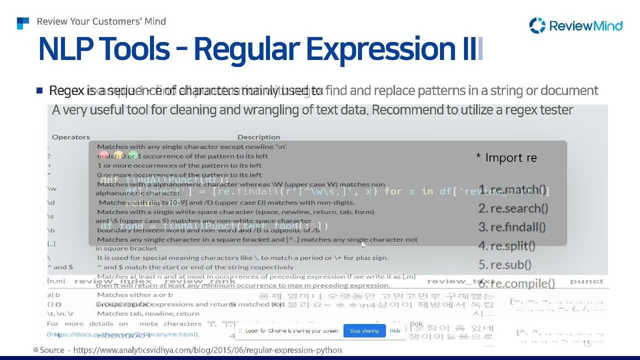 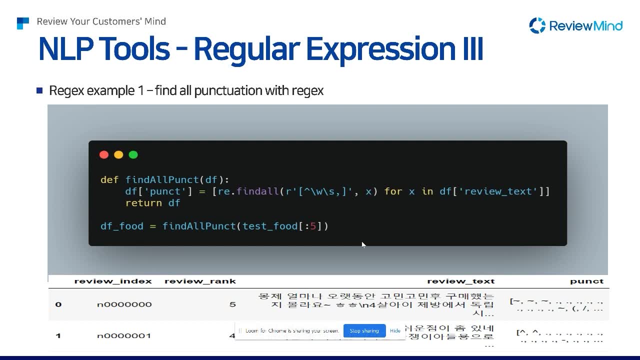 Let's check some use cases with regular expression. The most NLP preprocessing package, such as NLTK or spaCy, are also supporting regular expression. They are often used in the case of punctuation remover function, but in my case they were never enough in a real-world project somehow, so I had to handle some remaining erratic. 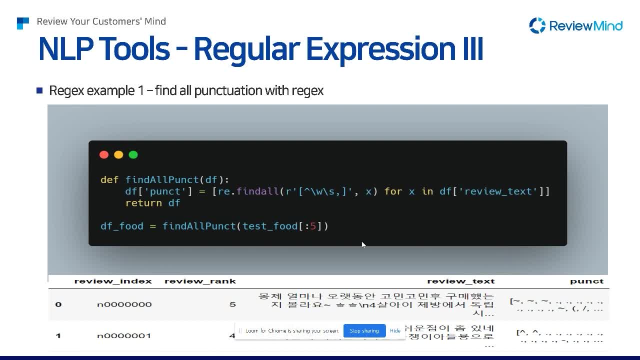 punctuation all the time using this regular expression. This Python code example shows how to check the punctuations in Korean text data. So in this regular expression's rules I tried to find punctuation. However, it was only effective if the punctuation was consistent with NLTK. 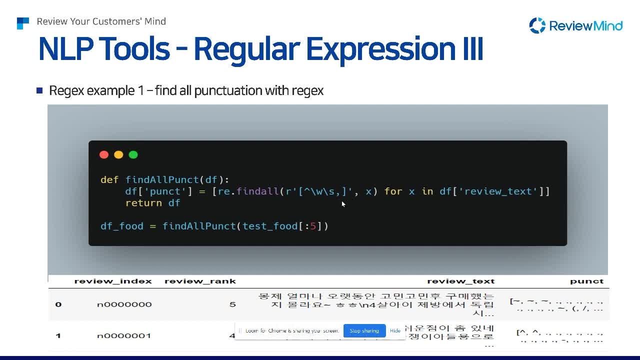 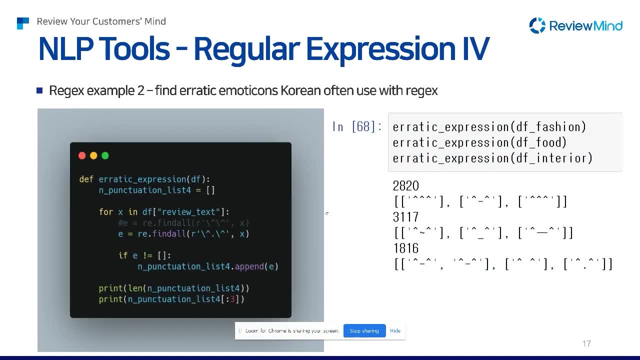 In this case I had to handle some remaining erratic punctuation all the time using this regular expression: every characters except a word or space. The other use case is telling you how your analysis domain can affect on your decisions, on how you're going to do the text preprocessing task. These are the special 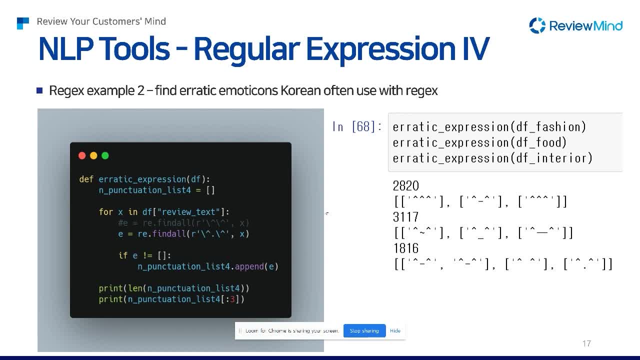 language usage of Koreans. very unique kind of language expressions, behavior: to express your emotions using some punctuation characters. It's like something like emoji In this case. maybe I need to identify them separately using regular expression and treat them like their corresponding emoji or words. It rely on the decision of 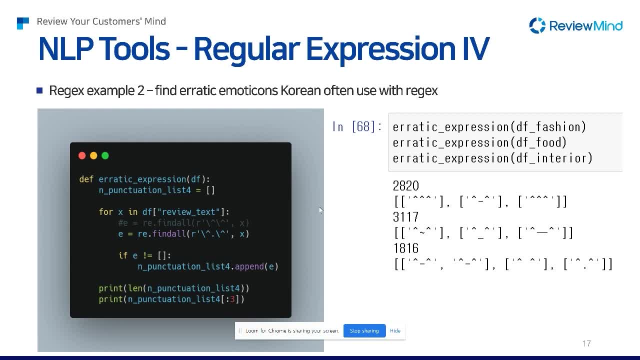 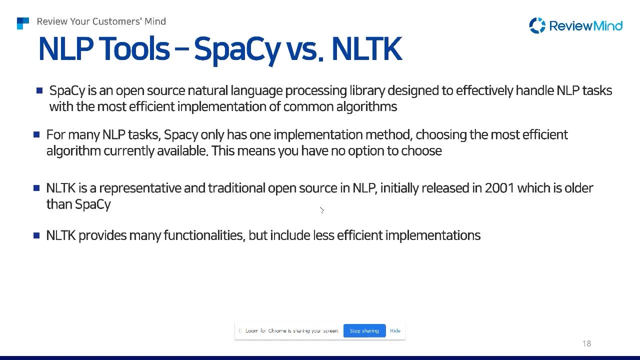 each data scientist. The next representative tools for NLP are NLTK and spaCy. Both of them are Python open source commonly used. spaCy is an NLP library designed to effectively handle NLP tasks with the most efficient implementation of common algorithm For many. 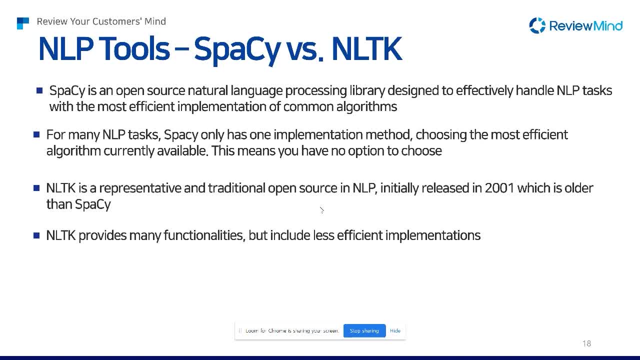 NLP tasks, spaCy only has one implementation method: choosing the most efficient algorithm currently available, which means you have no options to choose for your target NLP preprocessing task. Meanwhile, NLTK is a representative and traditional open source NLP toolkit, initially released in 2001,. 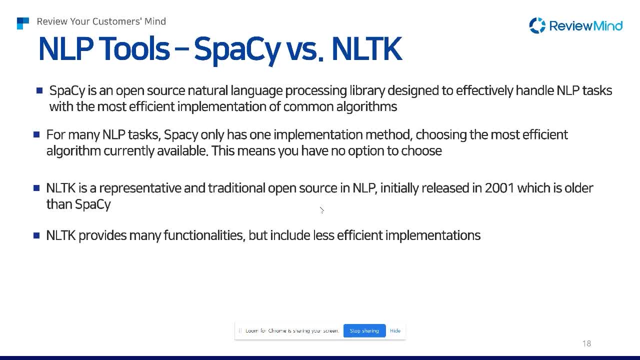 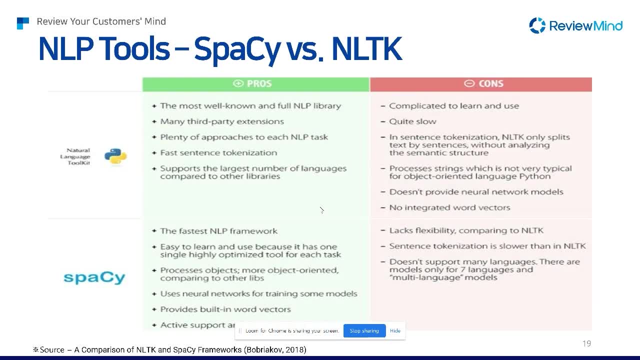 which is much more older than spaCy, But NLTK provide many functionality but include less efficient implementation usually. The table of this slide is showing you the comparison of these two most well-known NLP tools. It's mentioning that NLTK is good for extensions with other languages or different approaches. 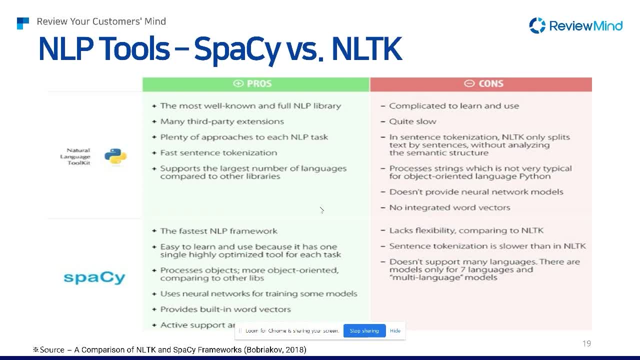 of each NLP task, while it's slow and a bit outdated for integrating with other NLP tools such as Word Vector. spaCy is the latest and updated tool, while its lack of flexibility and limitations of supporting language is mentioned as it flows. I personally have been watching. 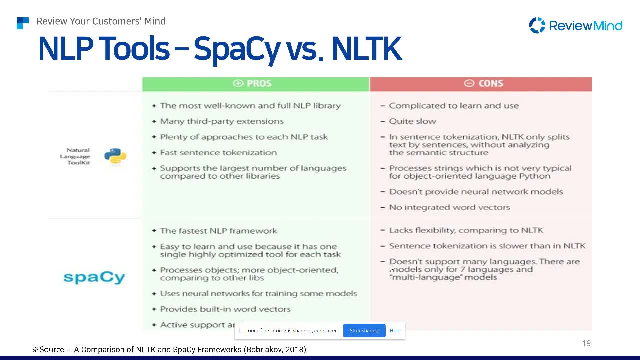 many recent big movements of spaCy. They are very interesting. Other than their fast updating open NLP toolkit, spaCy keep launching their new products, such as the integrated tool with transformer of Hugging Face or text annotation tools such as Prodigy. So I recommend you check their recent book. 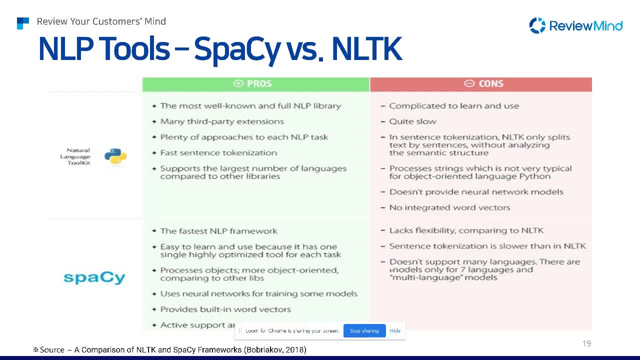 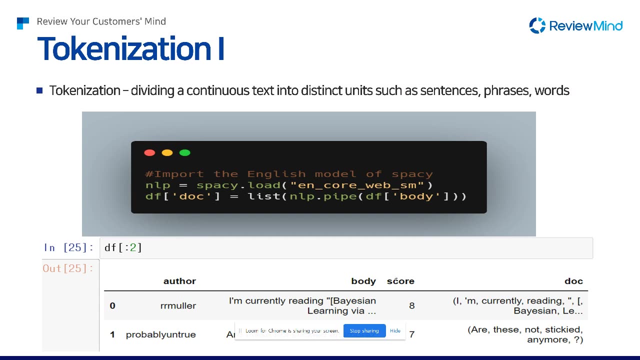 The book's name is the Mastering spaCy. It will be very helpful for your understanding and practicing of NLP text preprocessing task handling. Okay, then let's go back to the use cases of each text preprocessing task, The first of all. 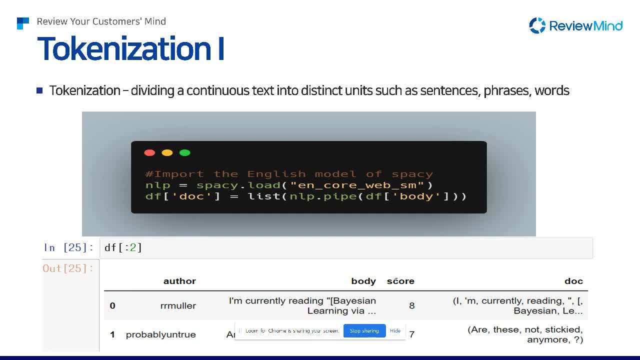 tokenization. Tokenization means dividing a continuous text into distinct units such as sentences, phrases or words, And this divided language unit can be a feature for the next computer analysis, like machine learning or deep learning. And it's usually a word in a real-world practice In this example. 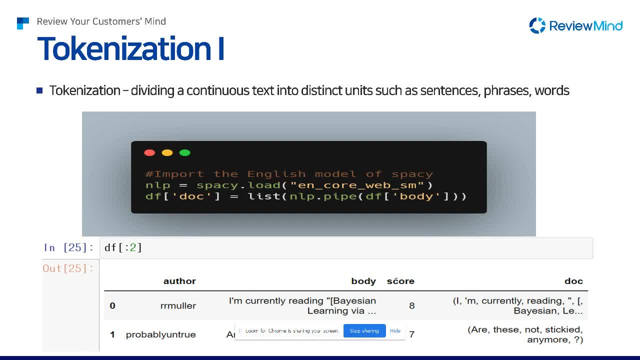 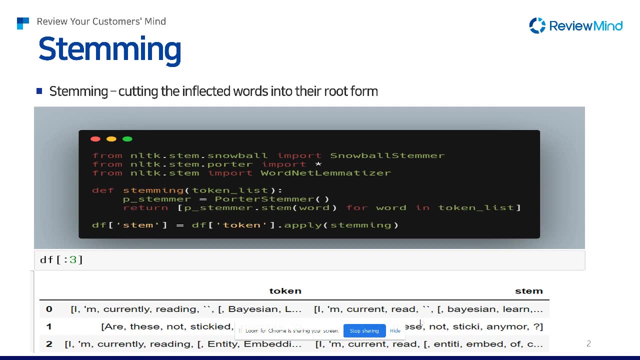 the both of tools, NLTK and spaCy have used white spaces- and tokenizes a text into the word analysis unit For stemming means cutting the inflected word into their root form, So all the verb or adjective or verb, past or present word will be. 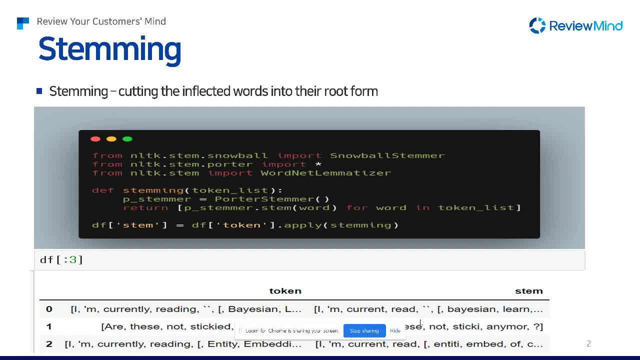 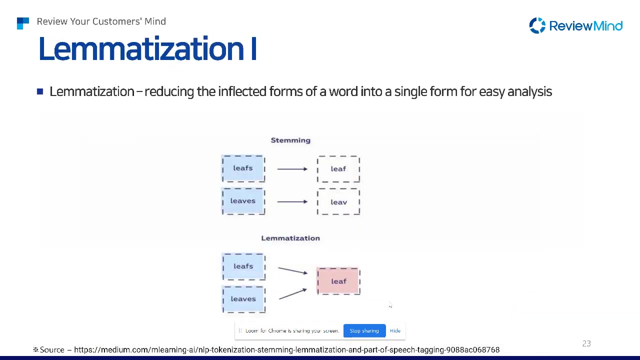 changes into their same root word. In this example, you can check. you can check the stem results of a few words like currently has been has been changes into current and reading has been changes into read and sticky has been changed into sticky, etc. Okay, the lemmatization means reducing the inflected form of a word. 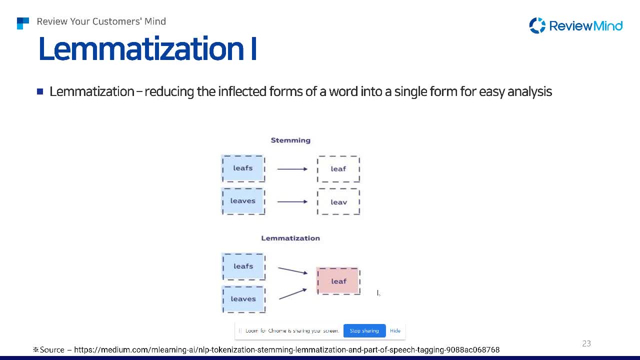 into a single form for easy analysis. Often stemming and lemmatization is confusing. So in this case, in this example, maybe make it clear for you. So in stemming, lived and leaves would be convergent into each different word as live and leave exactly irrespectively, But in the lemmatizations, 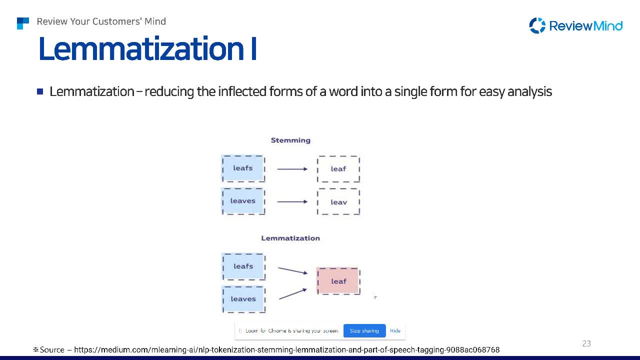 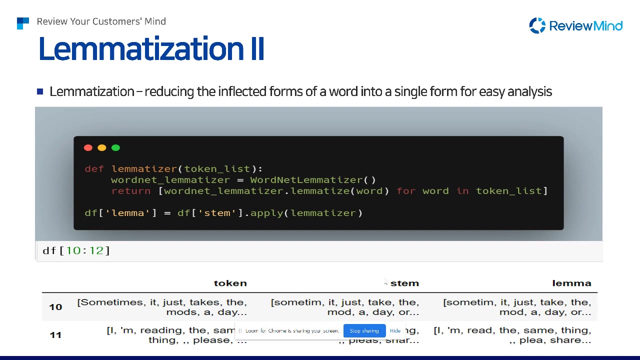 all of these words go to the one word leave. So it tries to make the word features into a more simple format by combining words into one root word in case they came from the same lemma. So it's a little bit hard to check the case in this example. 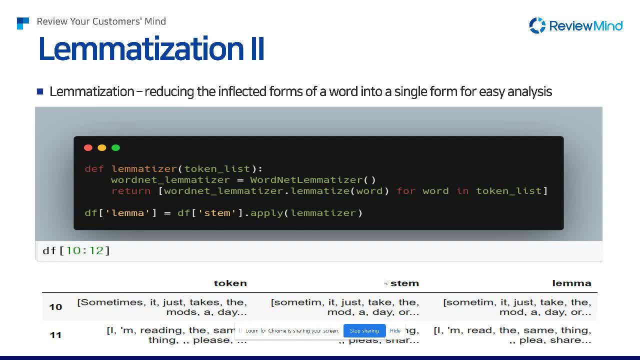 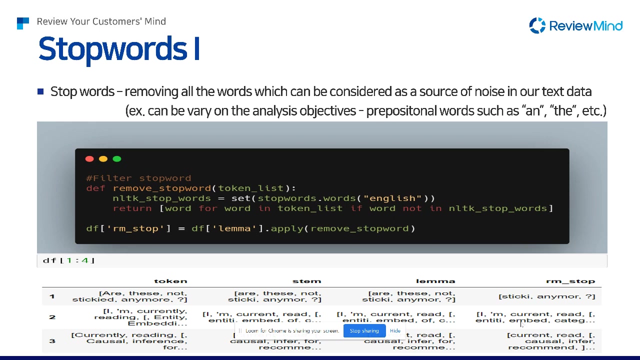 as they are mostly similar between stemmed and lemmatized results here, But you can check here. Please become PLEA plus S in stemmed result, But it became PLEA in the lemmatized result. Okay, next stop, word meaning. the words can be considered a source of noise in our text data. 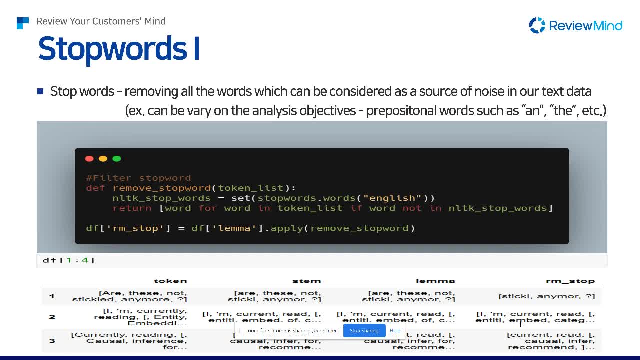 Usually it could be the prepositional words such as an, ON, D, etc. So in this example I have used the default English stop word from NLTK. The detailed stop word list from NLTK you can check in the next slide. 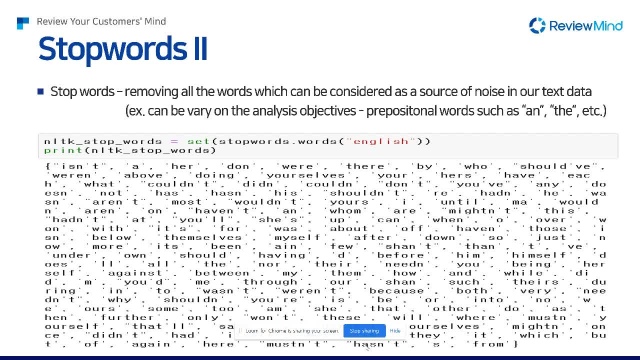 As you can see here, some negated words like isn't, are, not, are included in the list, But these negated words can be a very important feature in case you want to analyze the sentiment or complaint from the writer, depending on your target model. 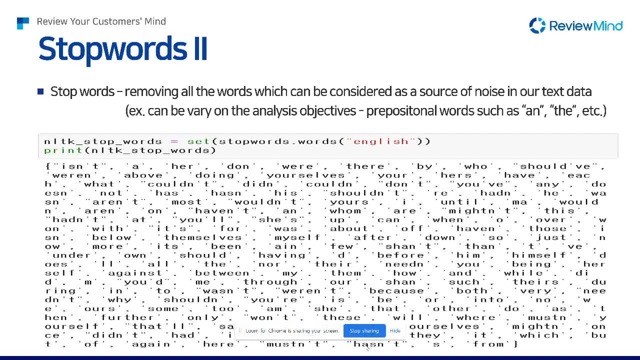 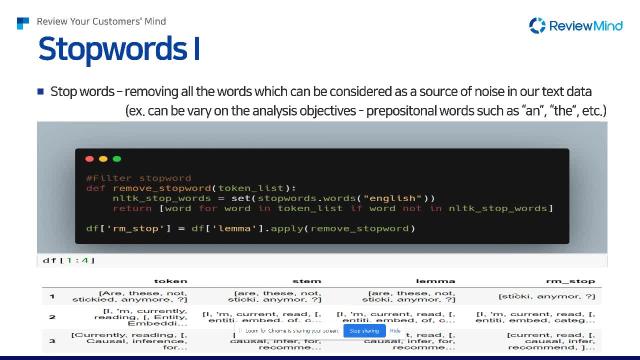 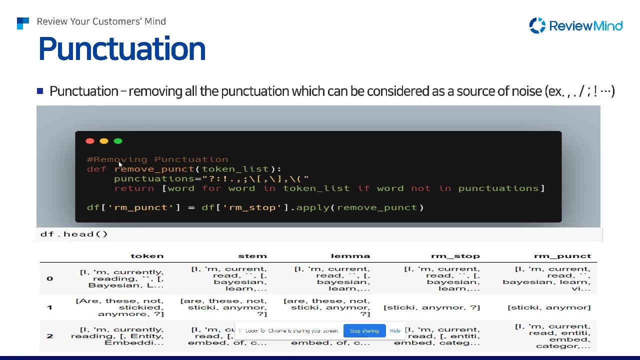 Thus, I recommend you should carefully check what you are removing in your analysis context. So in this example you can check the nots And these are this kind of words. These kind of words were removed after stop word removing. Okay, the punctuation also means the characters which can be considered as a source of noise. 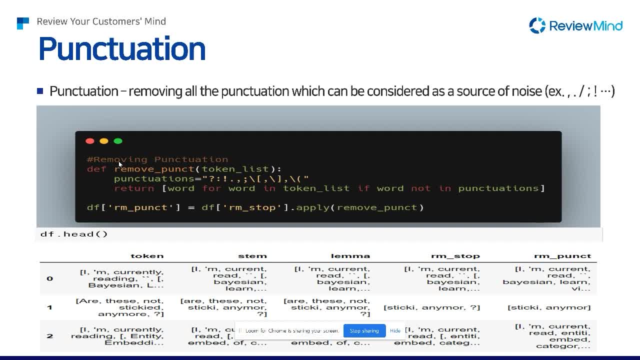 such as apostrophe, comma or the brackets, etc. You can observe here that the square brackets question mark were removed. I actually gave the punctuation list which should be removed using regular expression here. So the double apostrophe here were not removed, as it's not in the list. 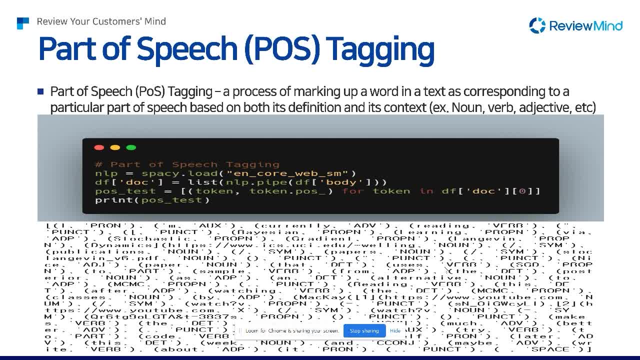 Okay, finally, power of speech tagging means the process of marking up a word in a text as corresponding to a particular power of speech, based on both its definition and its context, like noun verb objective. It can be helpful because POS is telling more clues about the rules of each word. 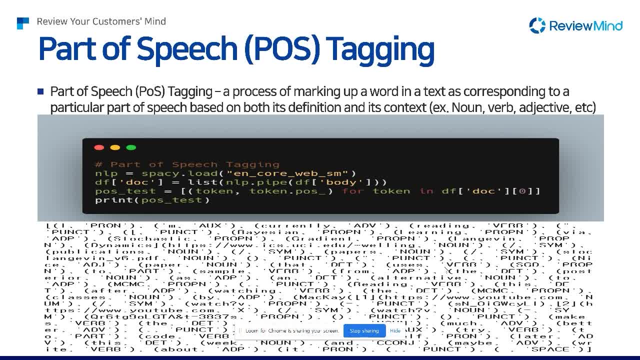 in the given text context. Usually in a sentence, noun and verb words can tell you more critical information than the propositions or interjection words, And you can utilize this information as the power of picture for your further modeling process. Okay, in this example you can check the results of POS tagging. 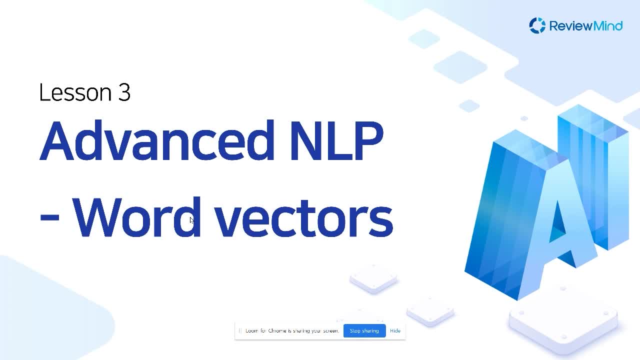 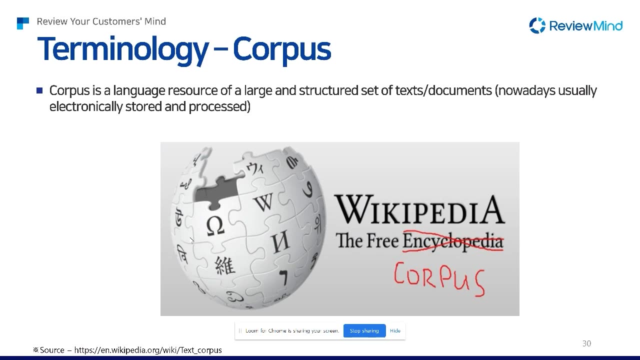 Using spaCy. here In this session we will talk about the more advanced NLP topic, which is word representation and word embedding. Before we go there, we need to understand the terminology of corpus first, as our further training or further analysis background will be really closely bound to the scope of your corpus. 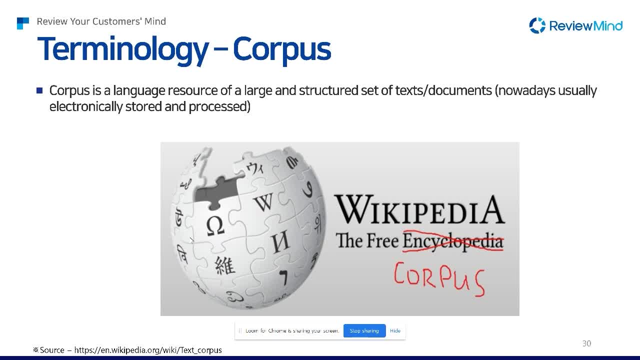 Corpus means a collected language resource of a large and structured set of texts or documents. You just can think Wikipedia would be a good example of corpus, and actually many companies like Google or Facebook are utilizing this as one of their NLP, research and development resources. 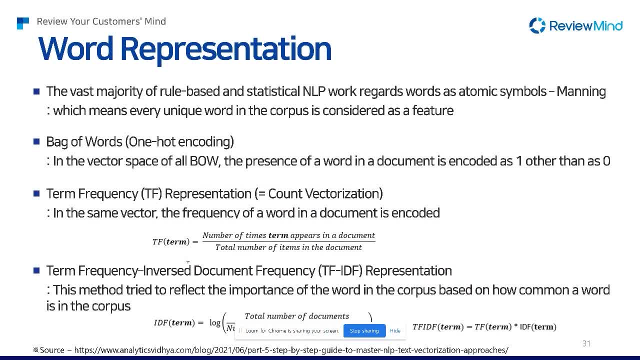 Okay then, what is word representation? Simply put, it is the way you feed your text data into a machine-readable format, and the best majority of rule-based and statistical NLP tasks regards word as atomic symbols, So you can enumerate all the words in your corpus as one vector. 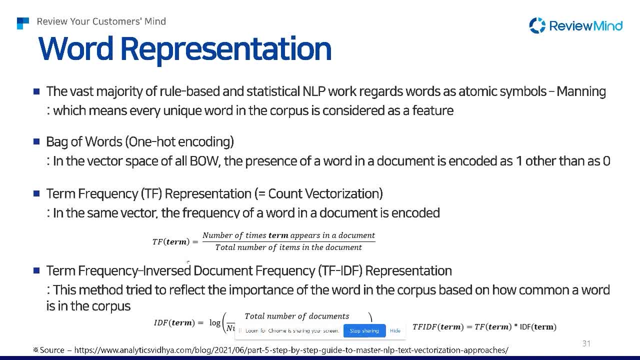 We call this as back-of-word, And you can describe each text document with the binary encoding of each word's existence. We call this in this case as one-hot encoding. From there, researchers have been studying a lot the way to more well describe this text document with a vector. 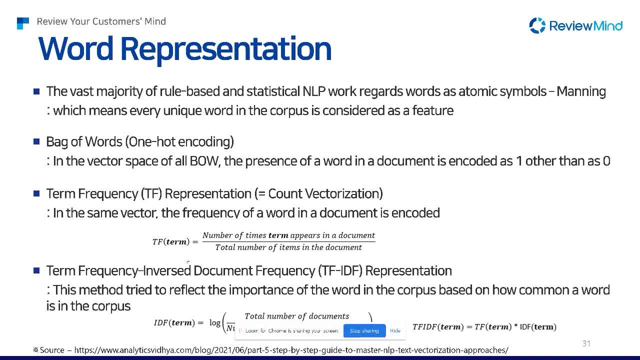 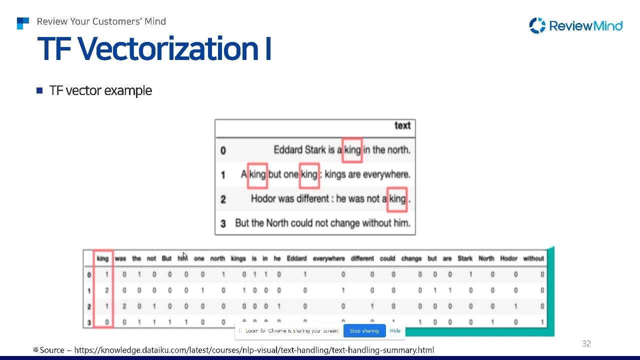 So its initial results are term-frequency representation, also known as counter-vectorization method, and TF-IDF representation. TF representation is simple: It's just the term frequency of each word, instead using the binary encoding of word's presence. So in this example, for the document 0,. 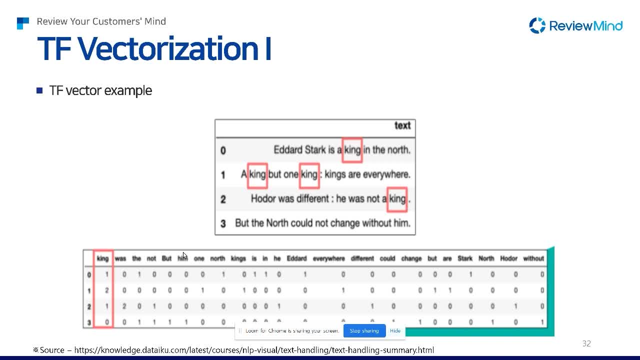 the word of king presents once, so the vector value of word king becomes 1,, while for the document 1, the word of king presents twice, so the vector value of the word becomes 2.. You can easily test this method using tools like sklearn or gensyn. 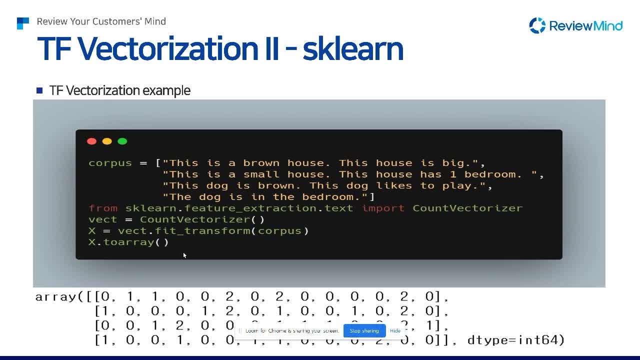 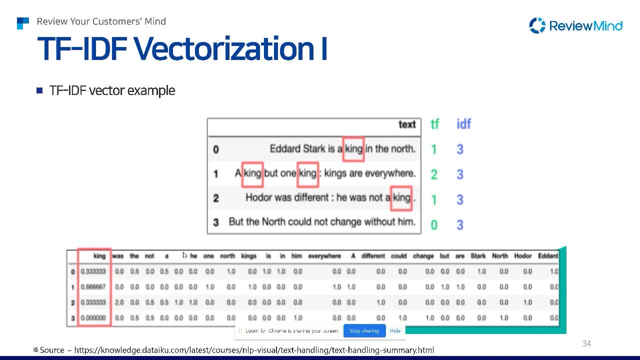 This is the use case with the word king. You can also test it with sklearn. TF-IDF tries to reflect the importance of the word in the corpus by multiplying TF with IDF, So the importance of common words such as A, D, etc. 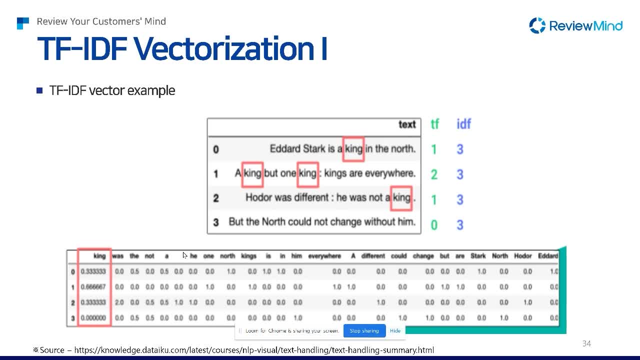 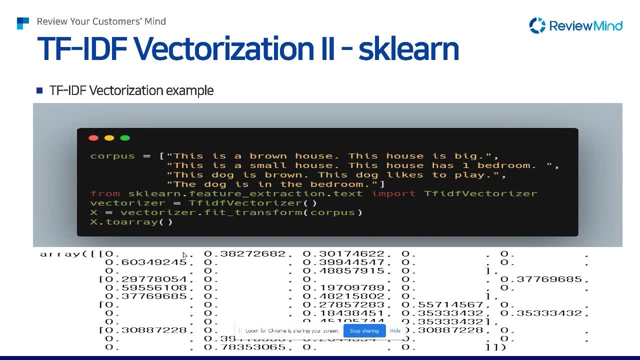 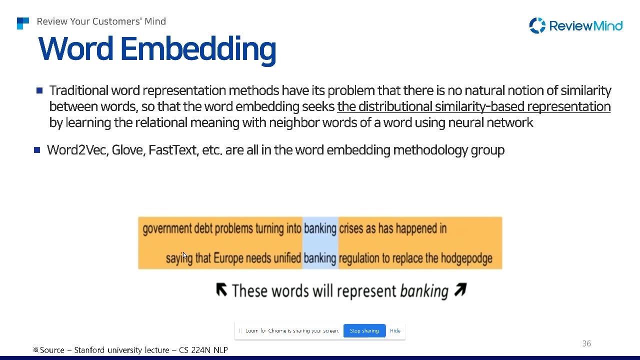 across the corpus can be evaluated in this function. You also can test this using the same tool. However, these kinds of traditional word representation methods have the problem that there is no way to reflect similarity between words, because they treated words as atomic units. So the concept of word embedding has emerged. 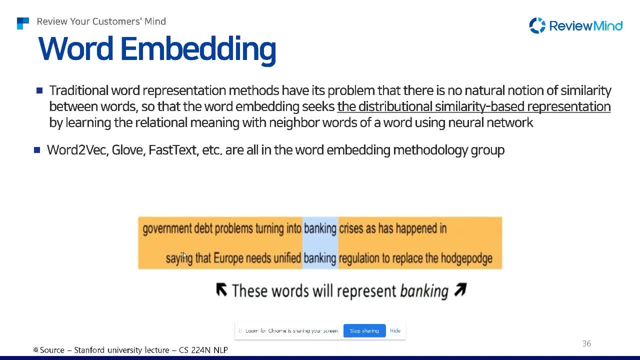 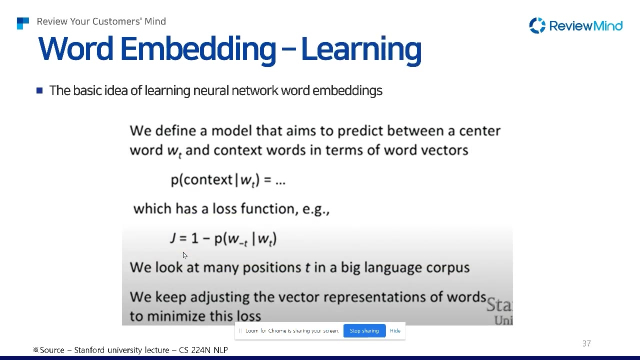 The word embedding is a distributional, similarity-based representation method by learning the relational meaning with neighbor words over words using neural networks. Therefore the word-to-back globe fast text, all of those are in the word embedding methodology group. The basic idea of learning neural network word embedding is 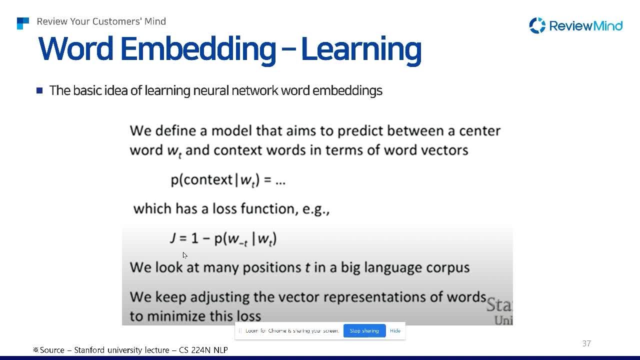 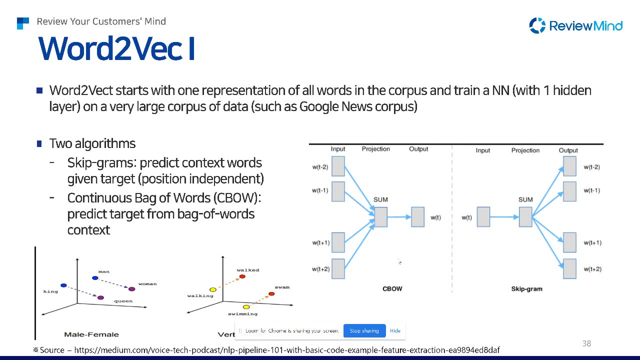 define a model aiming to predict between a center word and its context word in terms of word vector and keep adjusting the vector representation model to minimize this loss function. Then let's see the well-known word embedding method, word-to-back. Word-to-back has two algorithms. 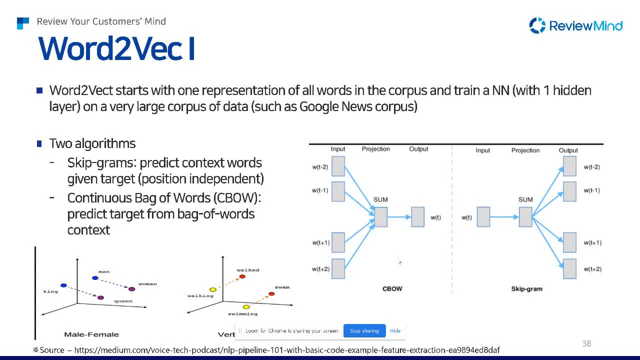 One is scriptgrams to predict context word based on a given target word and the other is continuous back-of-word algorithm to predict target word from the back-of-word context. You give the window size of context word, like 2 or 10,. 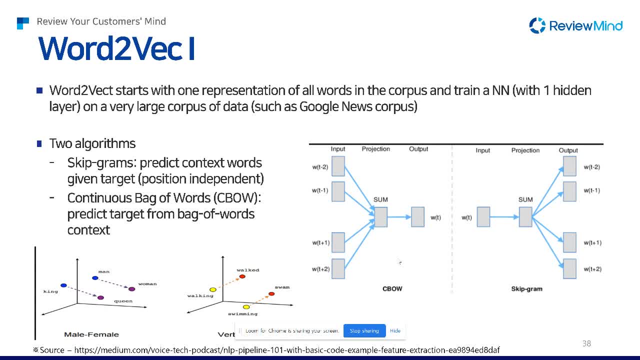 depending on your corpus domain. As a result, you can earn the trained vector value for each word and they can reflect some similarity between words, like this example in this graph Here. so you can see you can find some similarity between the men and women. 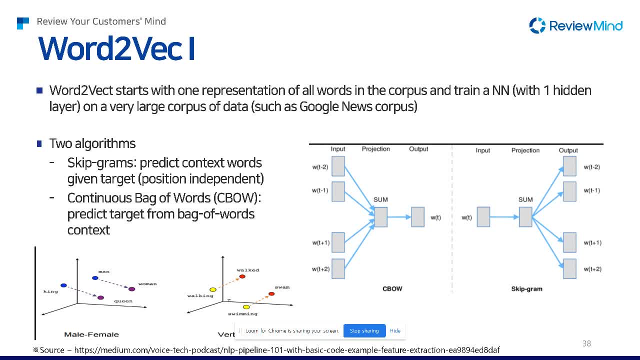 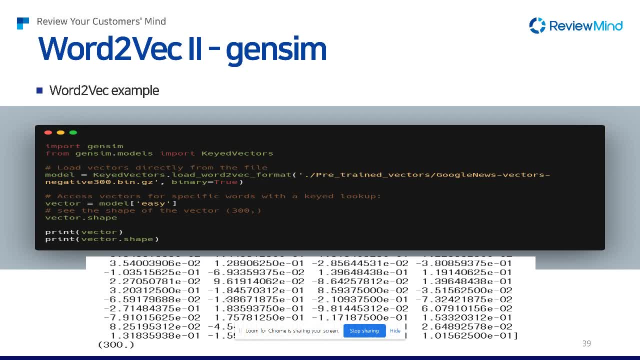 king and king, something like that. You also can test this method using GenSim or the other tools. In this example, I just extract the vector value of one word, which is easy, from the pre-trained vectors using word-to-back algorithm based on Google News Corpus here. 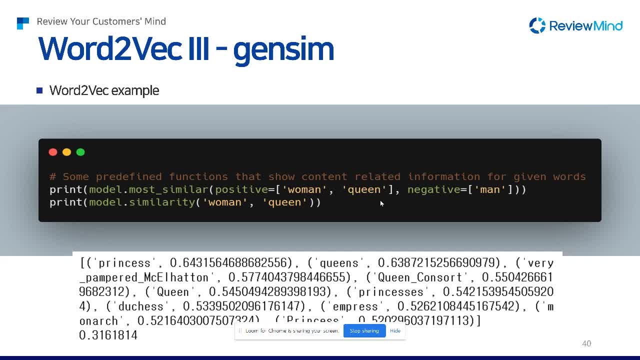 In the next example you can see how to check the similarity between words using the same tool here. So you can see you can find the most similar word with the women and queen positively, Meanwhile it's negative, it's far away from the men word. 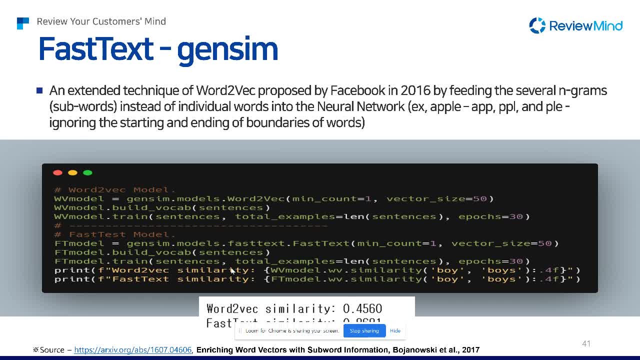 The FAST text is an extended technique of word-to-back proposed by FAST and it can be used in many ways. For example, if you look at this book in 2016,, this algorithm feeds several n-grams, which is sub-words of individual words. 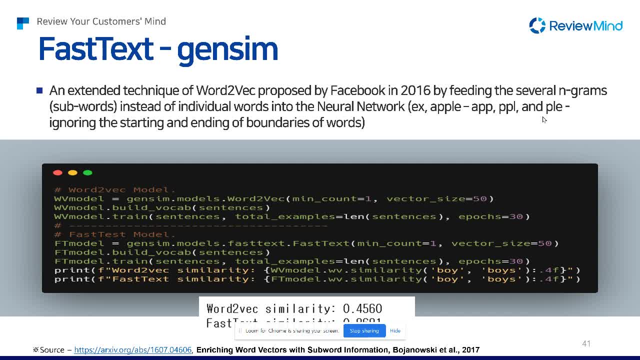 into the neural network. For example, you feed F, PPL and PLE instead of one word of apple. It is reported that FAST text can handle auto-vocabulary words much better than the word-to-back, and it's useful when you don't have. 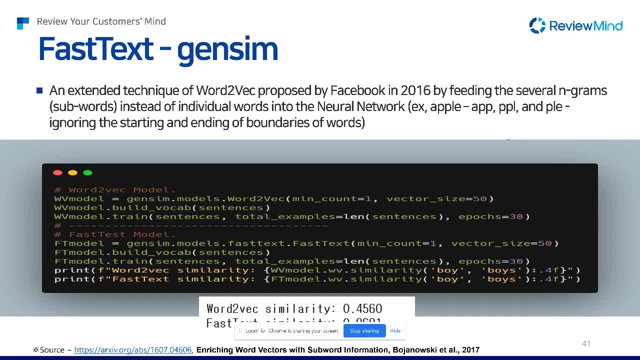 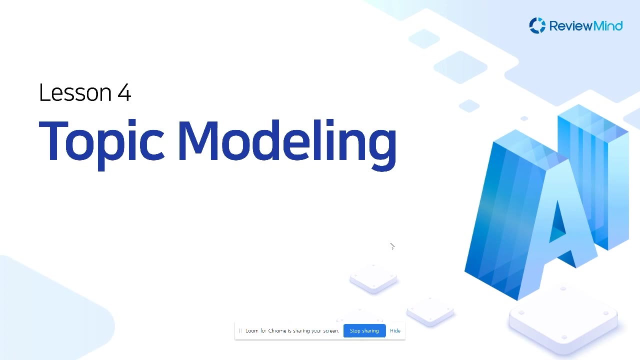 enough big size of corpus. In this small-size corpus training example you can check that FAST text shows better similarity results than the word-to-back here when you give the query: the similarity between the boy and the boys. Finally, we left the one last session. 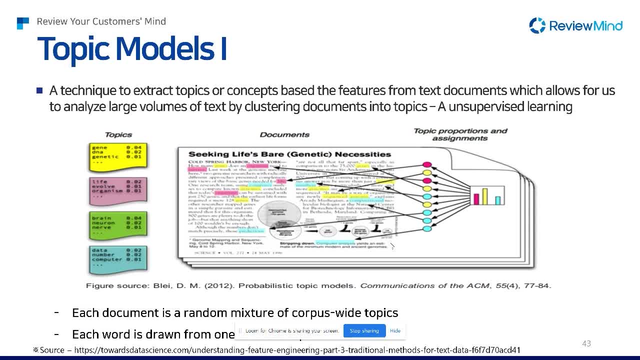 which is topic modeling. Topic modeling means a technique to extract topics or concepts based on the pictures from text documents, which allows for us to analyze large volumes of text by clustering documents into topics. This is one of the unsupervised learning methods. It is a useful technology. 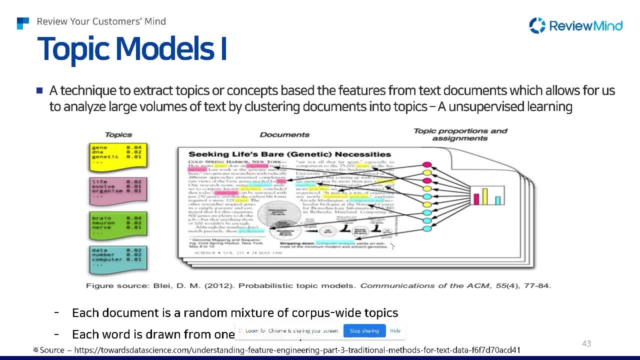 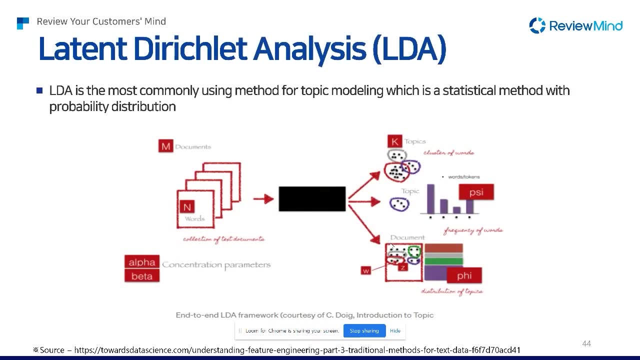 when you have an enormous volume of text or document resources, including important insights such as knowledge systems, and you need to cluster and classify them automatically in a more useful way. The most well-known algorithm in topic modeling is LDA. Its full name is: 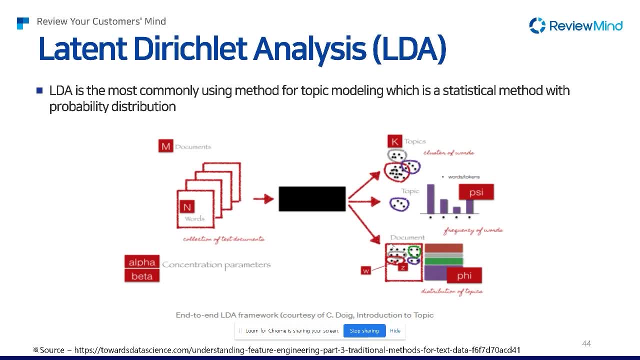 Latent Dechalet Analysis, which is a generative probabilistic model where each document consists of a combination of several topics and each term or word can be assigned to a specific topic. Each latent topic contains a Dechalet prior over them. 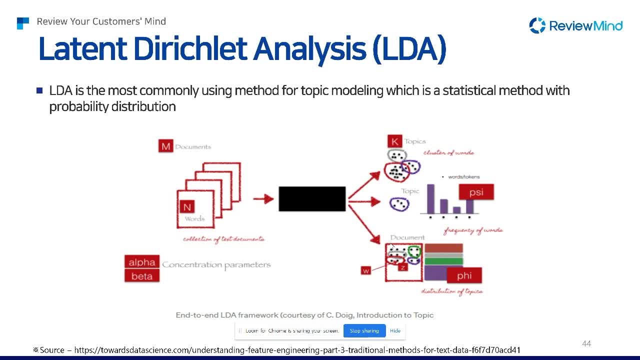 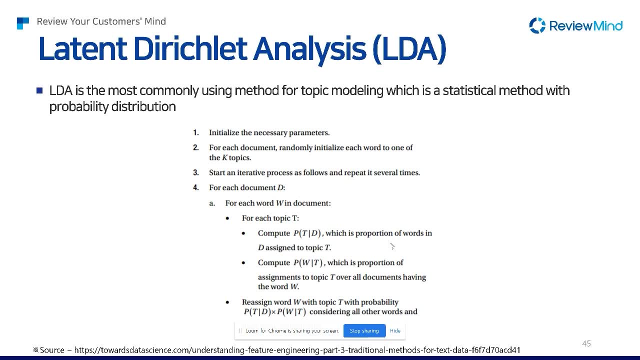 as it's based on the Dechalet probability. You have to decide the number of topics as its model parameter and it often gives a big influence on the coherence results of the word from each topic. You can test this LDA method using Gensim also. 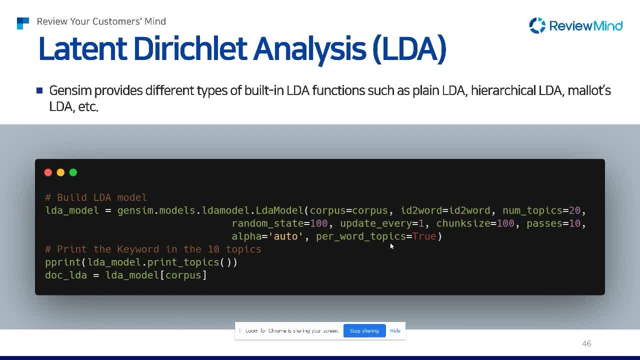 Gensim is a really good tool for this LDA, as it's providing different kinds of LDA algorithms, such as Hierarchical LDA, Merlot LDA, as well as Plain LDA. When you set the LDA model parameter like this code here: 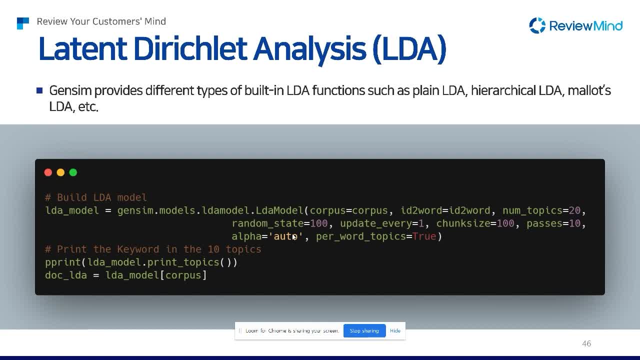 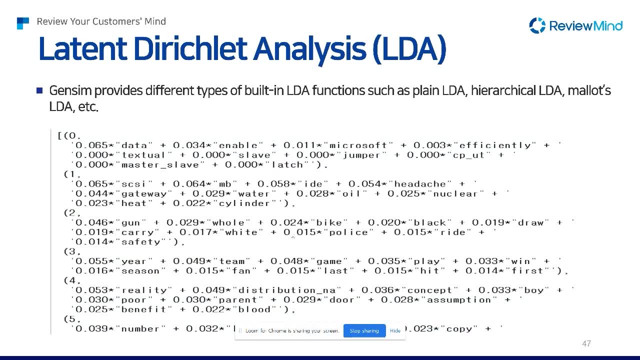 and run it based on your corpus. then you can run a LDA model like the next slide, which is expressing each topic with the keywords and their weight, Based on the. in this example, when you look at the topic zero, you can observe: 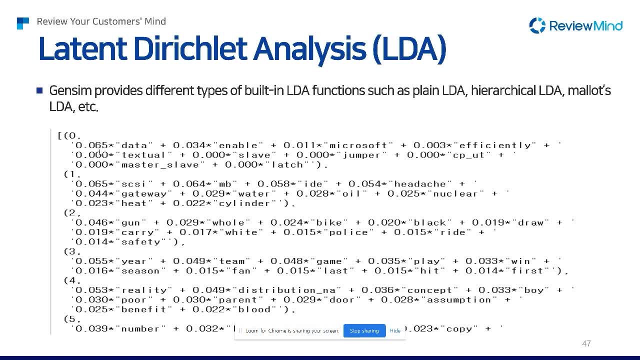 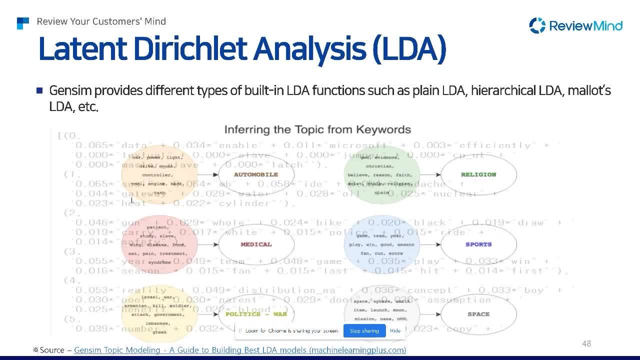 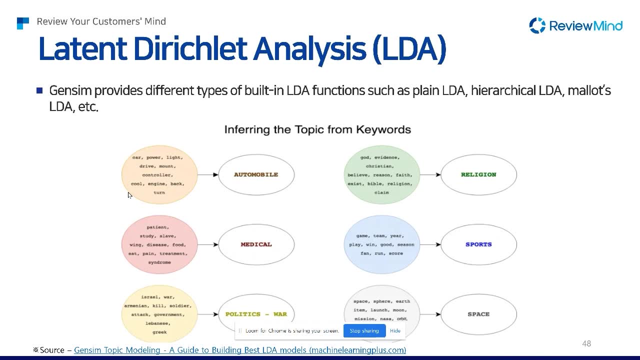 every keyword here related keyword and the weight according to each word. Based on the above model results, we can get some idea how this model is describing a topic with each related keyword, like this figure Here: the car power lights. 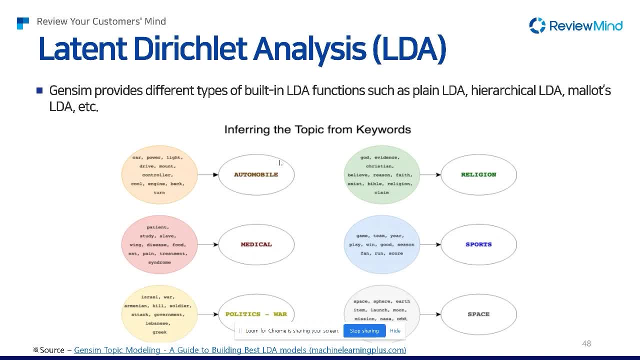 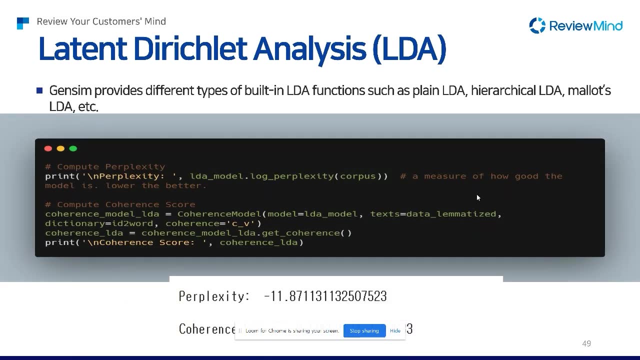 drive this kind of word describing this automobile topic. The good evidence Christians believe. this kind of words are describing this religion topic. One of the really useful thing of this LDA algorithm: you can check the performance of your model with the metrics of perplexity and coherence score. 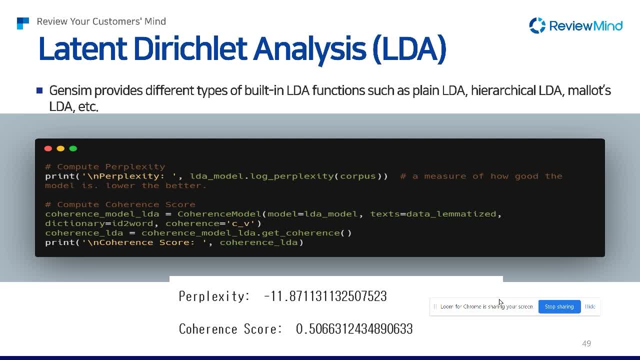 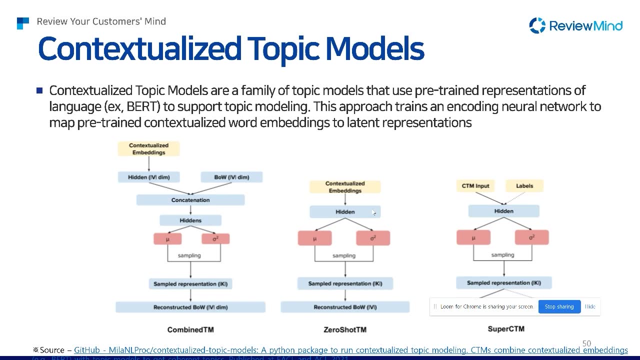 And you can try to adjust or optimize your topic model based on those metrics. In my experience, especially the coherence score was useful to find the optimal number of topics. In our recent research field, this topic modeling methodology is evolving, or so by trying to embrace 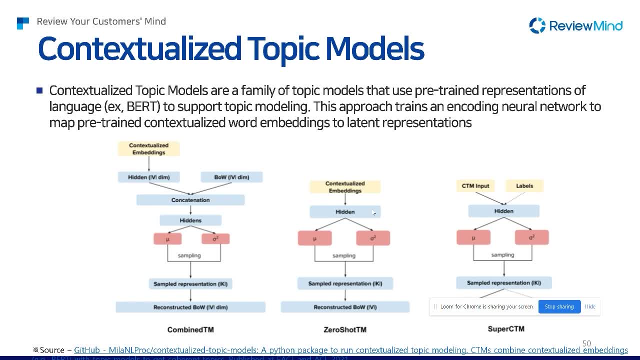 the benefits of pre-trained neural network language models like BERT. So the contextualized topic models become a new innovative approach in this NLP category, NLP task category. In this approach it's good that you can- you also can utilize the visualization tool. 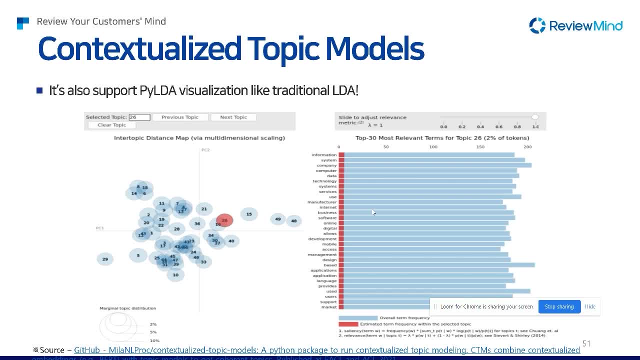 of PI LDA like traditional LDA, as you see this figure in this figure. I just mentioned this new approach to let you know the technical trend in this NLP task category, So I will not go further for the detail of this approach here. 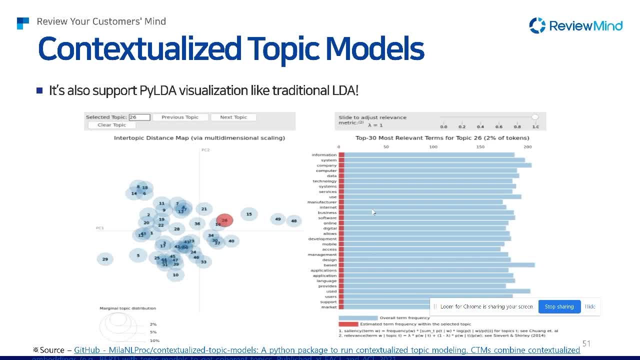 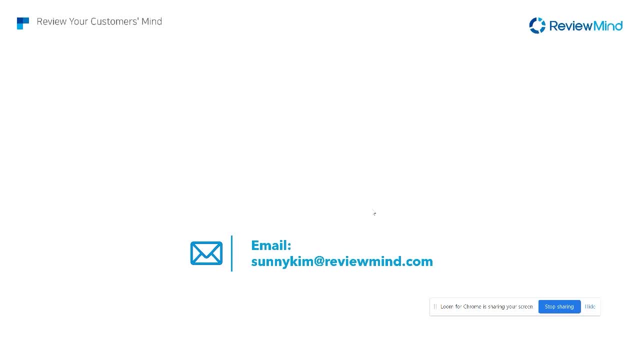 and recommend to check the paper or its GitHub repository if you are more interested in this topic. Okay, then let's call today's talk session. Thank you for listening to my talk session. Hopefully I can meet you guys in person in the next opportunity.